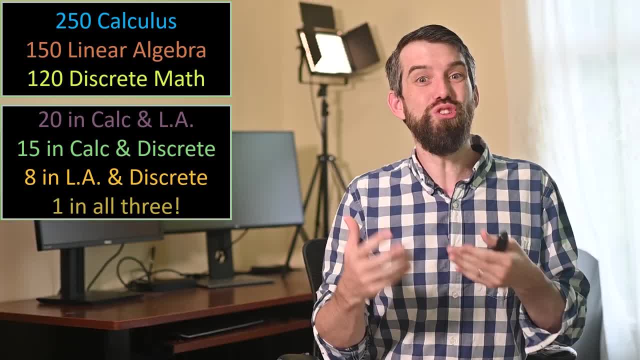 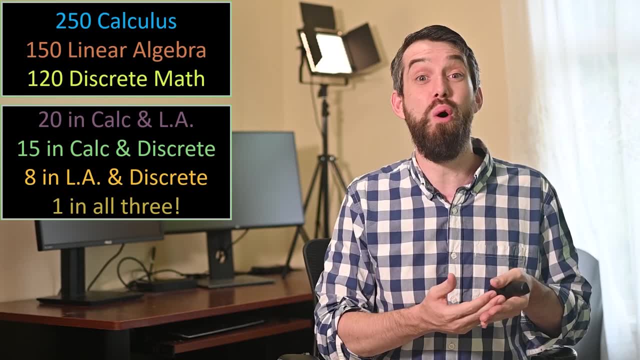 That student's definitely Going to have a lot of fun with me this summer. So I actually have seven numbers here: the three numbers for the total, the three numbers for what I'll call the double intersection, So that students who are in two of my classes 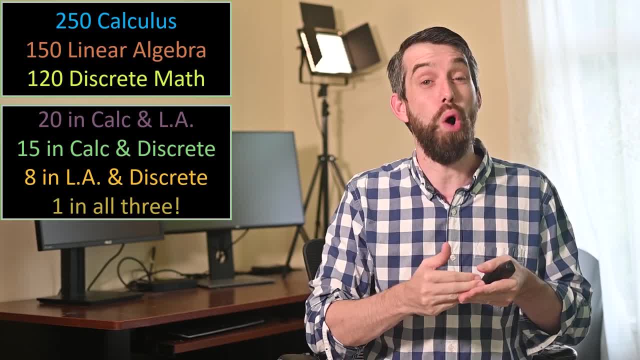 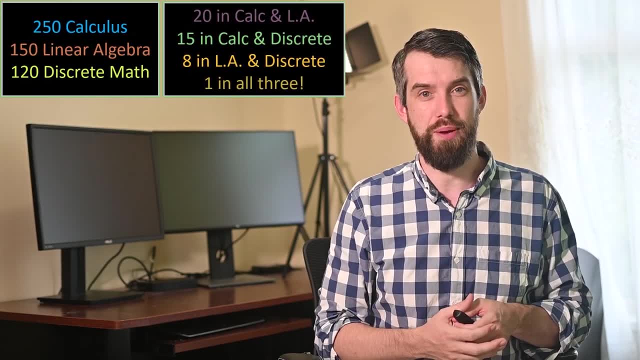 and then I have this one final piece of data for the student who's in all three classes at the same time. There's a great pictorial way to visualize this: with Venn diagrams. Here's the idea: These circles represent the calculus students, the linear algebra students, 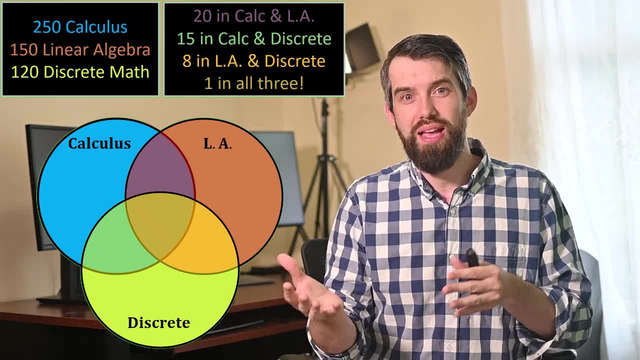 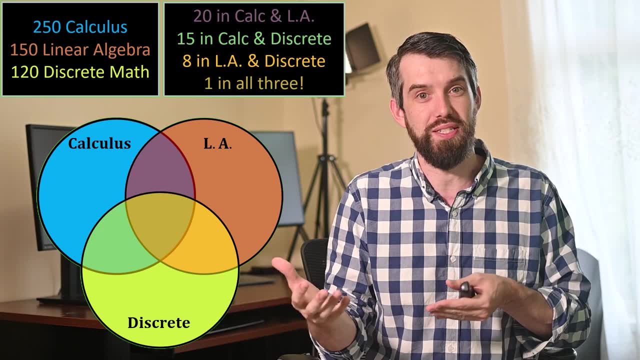 and the discrete math students respectively, But they overlap, and the overlaps between them indicate students who are in both of the two courses, or all three of them at once, And so what I'm going to try to do is basically fill in this so-called Venn diagram with appropriate numbers. 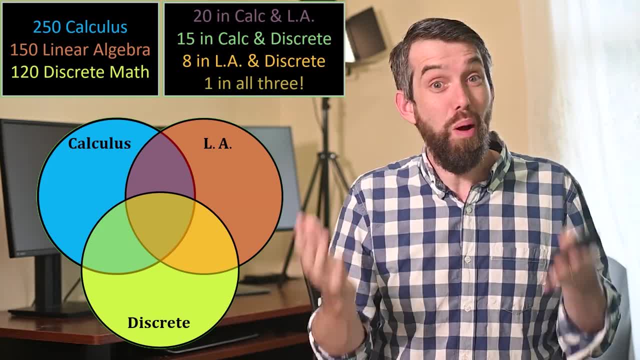 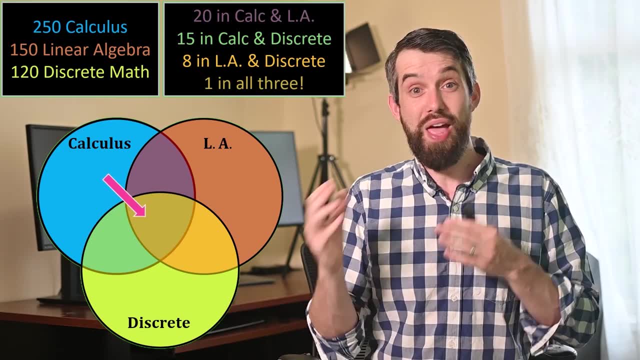 And I'm actually going to work from the smallest numbers out. The smallest one is the triple intersection: the student who's in linear algebra, who's in discrete math and who is in calculus, who's in all three of them. So that student belongs well right in the very middle. 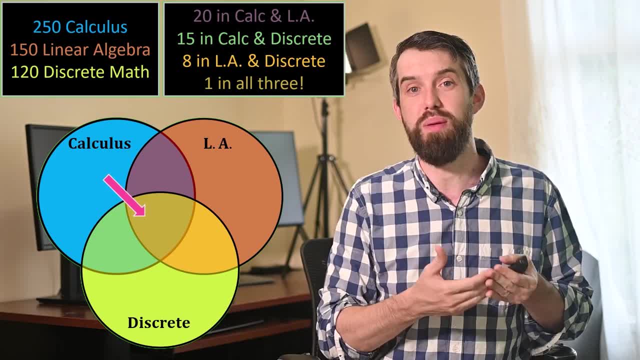 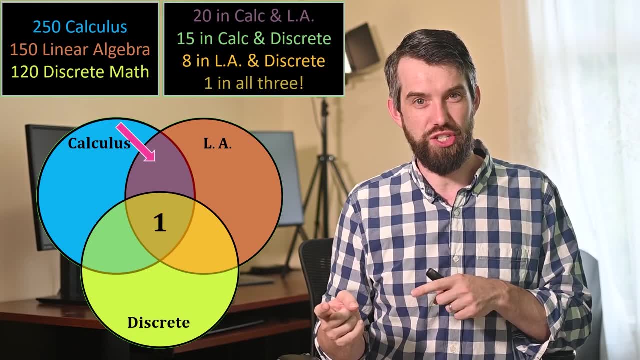 that is where the overlap between the Calculus, the Linear Algebra and the Discrete Math is, And so I'm gonna put that one student right there and fill it in with the one, Okay, so the next thing I want to look at is this next region. So 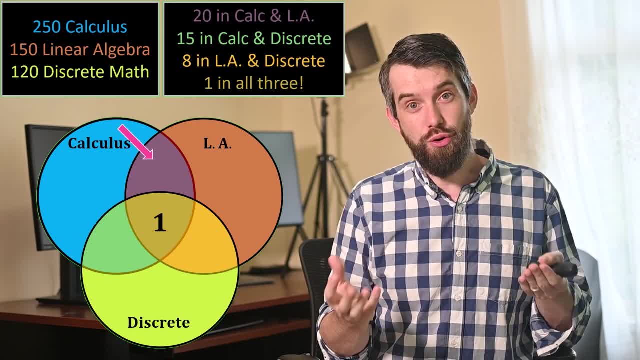 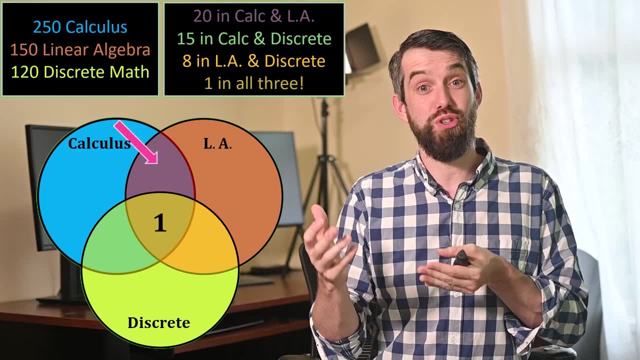 this denotes the students who are in Calculus and Linear Algebra, who are in both but who are not in Discrete Math. I left the triple intersection Okay, so what number should I put in here? Well, I know there's 20 students in Calculus and 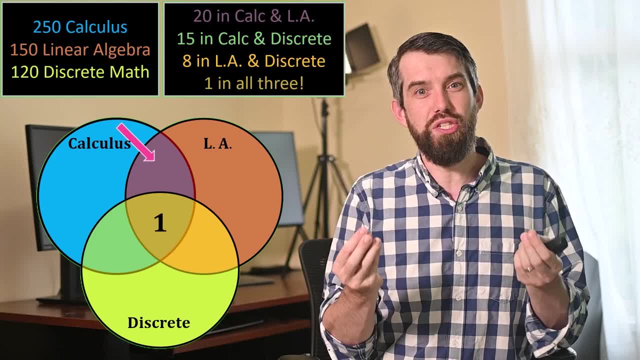 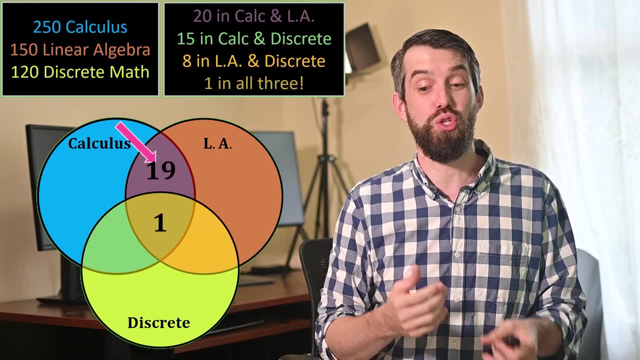 Linear Algebra in general. However, of those 20 students, one of them is already accounted for, One of them is in all three, So that actually means there's only 19 students who are remaining: The 19 students who are in Calculus and. 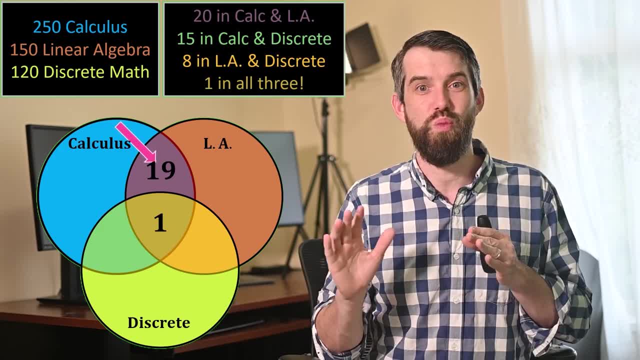 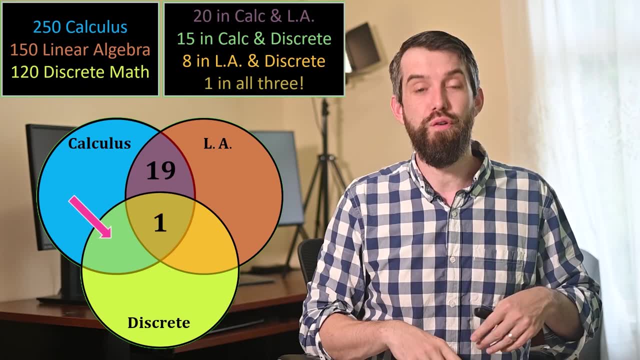 Linear Algebra, but not in Discrete Math. Okay, wonderful, Let's maybe move on to the next of these double intersections. So these are students who are in Calculus and Discrete Math, but not Linear Algebra. For all of Calculus and Discrete, there's 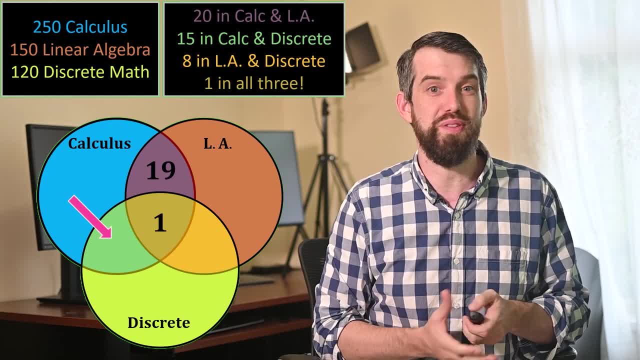 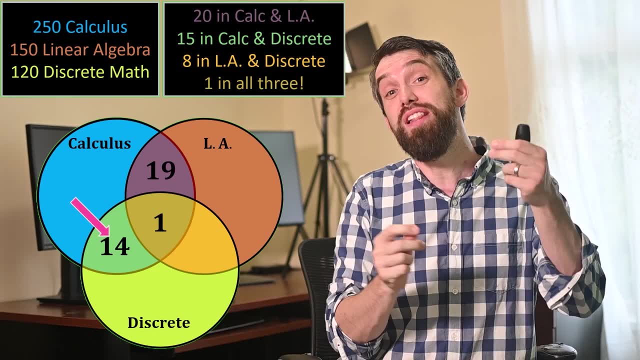 going to be 15 students. One of them is already in the triple intersection, so I have to subtract that out and that gives me just 14.. I'm actually going to encourage you at this point to pause the video and see whether you can just fill in all the different locations in this diagram. 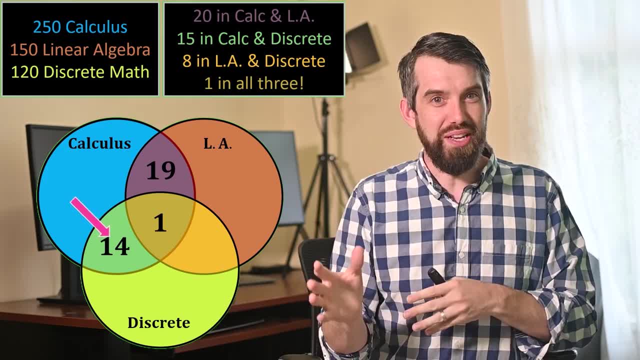 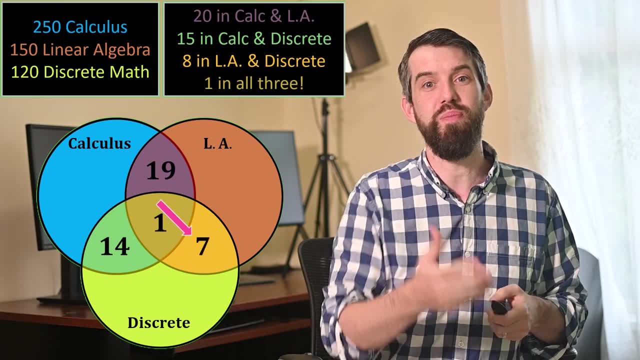 yourself. If you've managed to go and do that, then great, And if you're just here to watch the show, then well. the other double intersection- this is the 8 people minus 1- is just going to be 7.. And then I've got the three outsides, like: 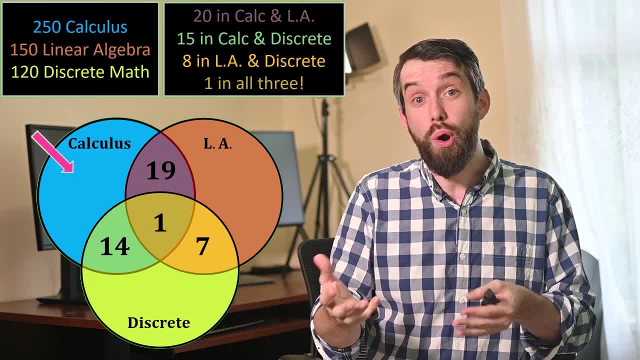 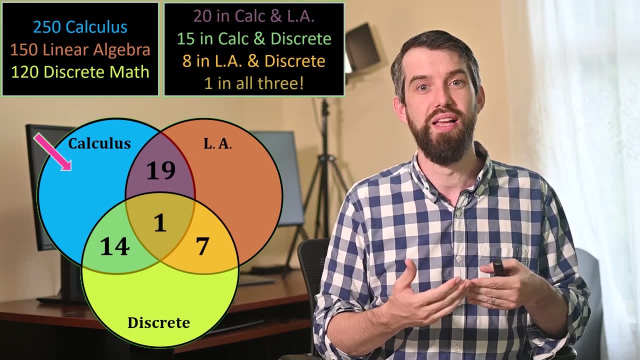 for example, the portion that are in Calculus but not in Linear Algebra or in Discrete Math. I have 250 to start with, but that's going to be subtracted off the 19 plus the 1 plus the 14.. So I'm taking the 250, I'm 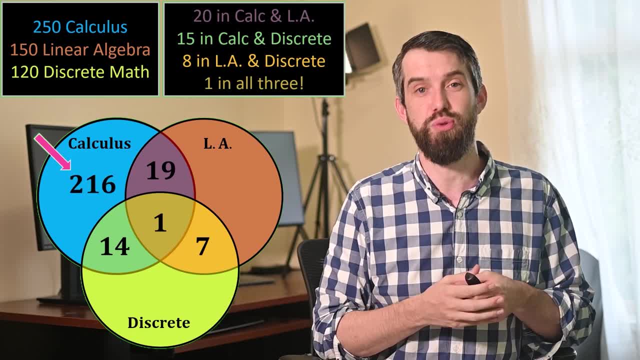 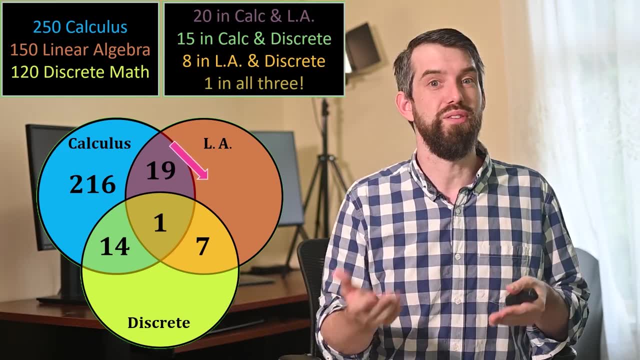 going to be subtracting the 34,, I'm going to get 216. So this is my result: 216.. So again, these are students in Calculus, but none of the other courses. Same sort of story for the Linear Algebra. there's 150 to begin with, there's 19 plus 1 plus 7, which is 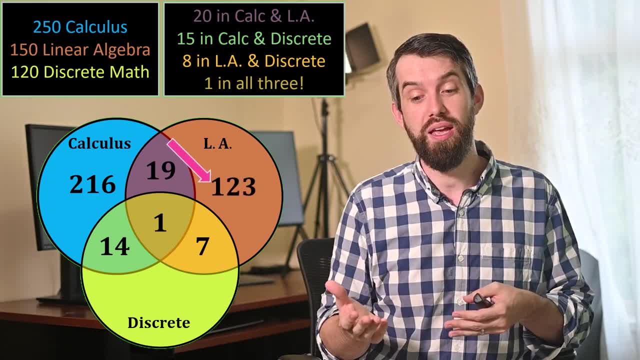 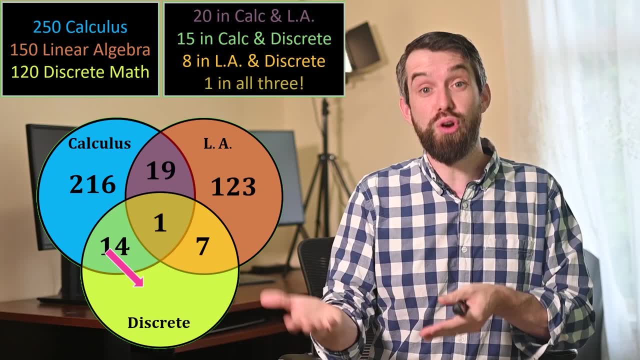 27 already used up and that leaves 123 remaining. And then the final one is: how many Discrete students are there? Well, there's 120 Discrete students total. there's 22 of those are in some other courses, with just 98 students to fill here. So what I've done here is I filled out all the possible places. 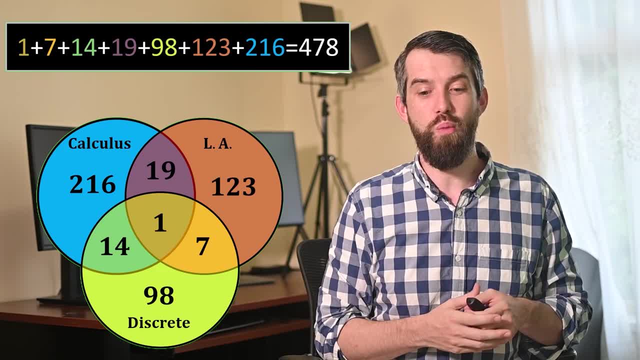 in this Venn diagram, And now I can get an answer. If I want to figure out, well, what is the total number of students, I just add up all these numbers. add up the 1,, the 7,, the 14,, the 19,. 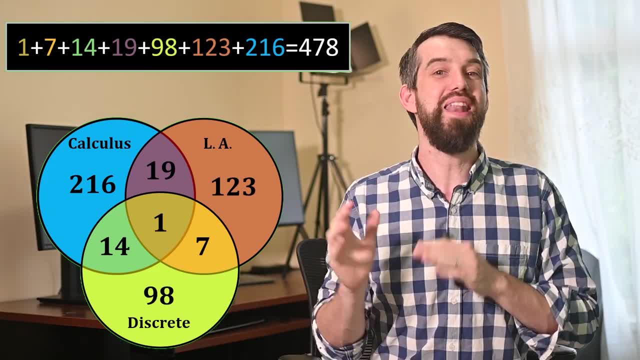 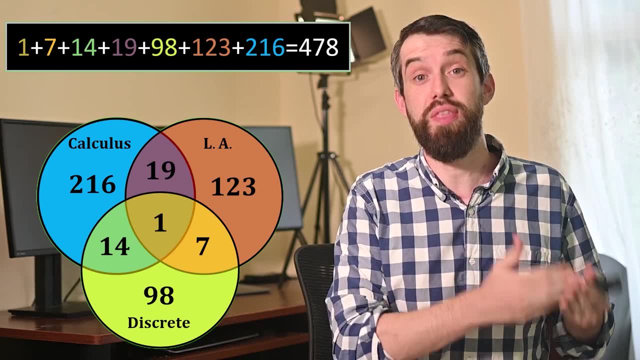 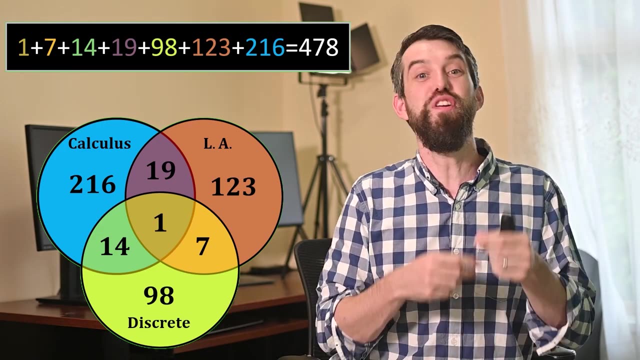 the 98,, the 123, and the 216.. And I added that up and got 478.. So that's how many individual students I am teaching this semester. So that's one way to answer these kind of triple intersection arguments. You write down the Venn diagram, You try to figure out like what numbers go in each. 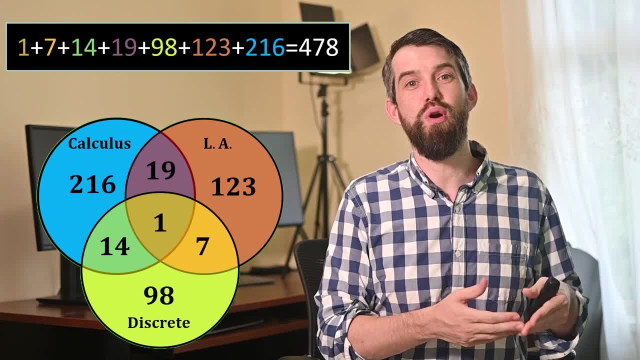 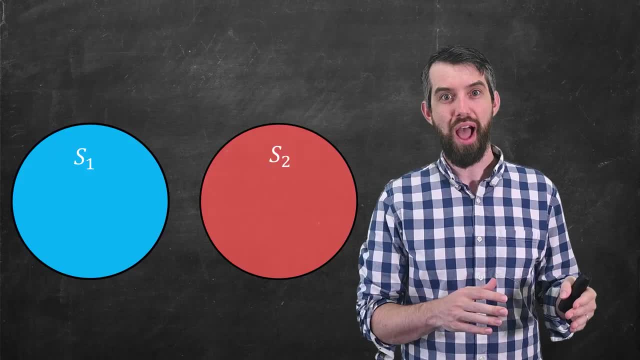 possible region in the Venn diagram. I also want to show you a bit more of a formulistic way to do it. We're going to come up with a generic formula for the triple intersection. Moving over to my chalkboard, I'm actually going to begin now by just considering two different sets, And I'm 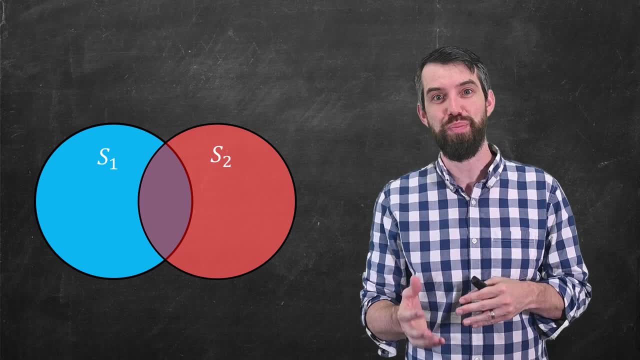 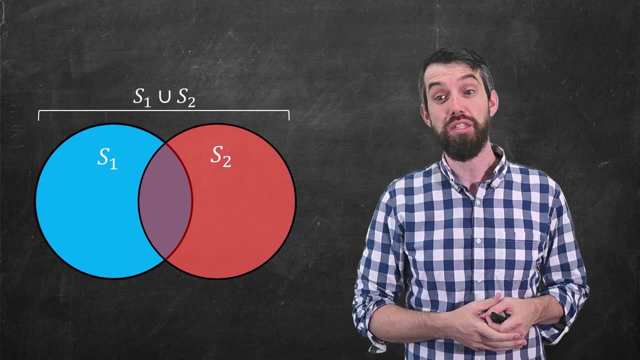 going to imagine that these two different sets- S1 and S2, are overlapping, which means that there's some intersection in the middle. Now, the terminology that I use here is: I use the union symbol S1 and S2.. And I'm going to use the union symbol S1 and S2.. And I'm going to use the union. 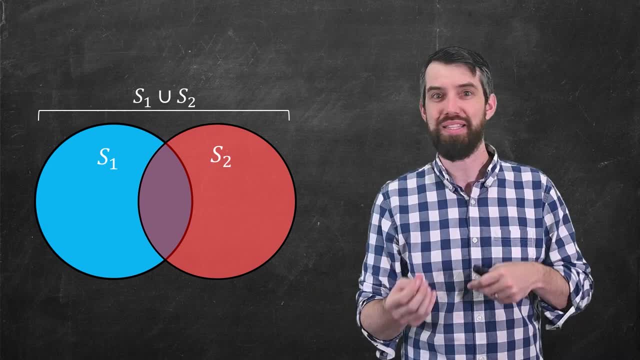 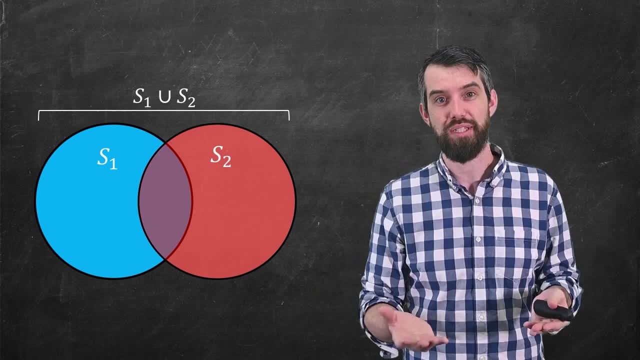 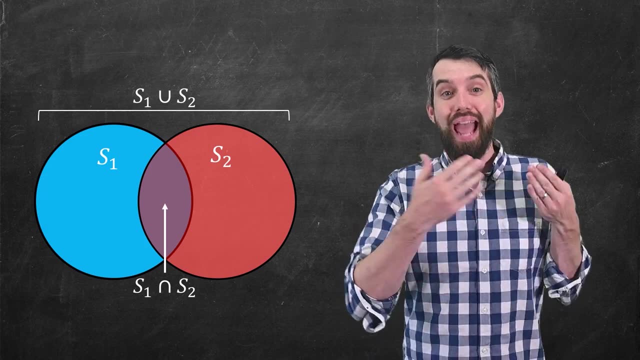 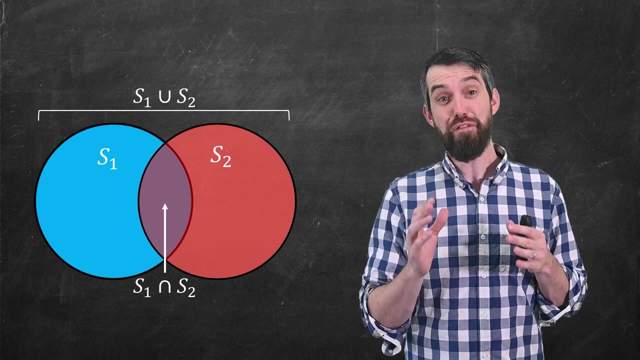 if an element is in one or the other. That's what the union sign means. And then the intersection sign that looks like an upside down U. it means for elements that are in S1 and S2.. So unions sort of associated with ors and intersections associated with ands. So then my formula for: 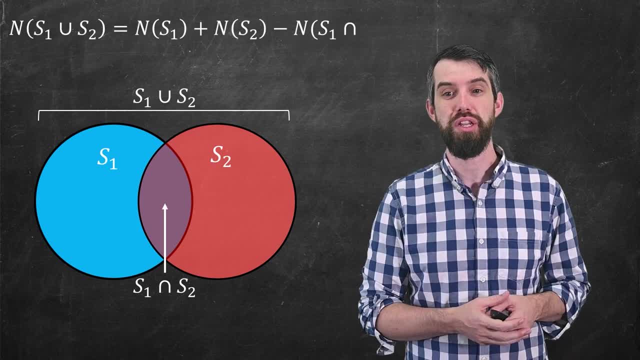 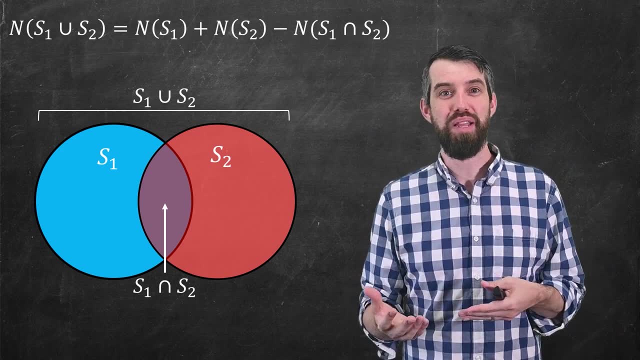 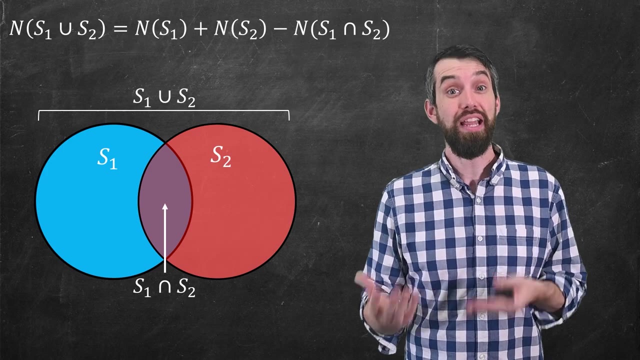 the number of elements in, well, the entire union, the S1 union, S2,. is this formula here Okay? so what's going on with this formula? So, first of all, by n I just mean the number of elements in a particular set. So the number in S1 union, S2 is just read in English as the number. 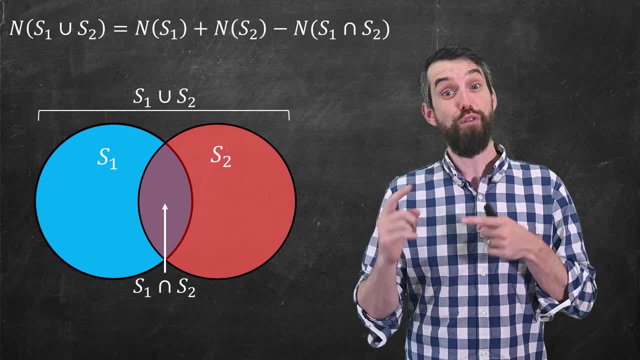 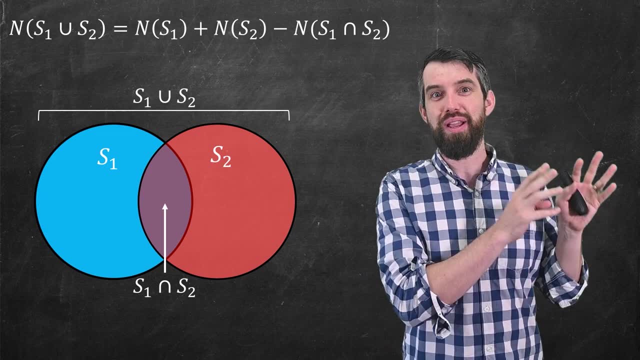 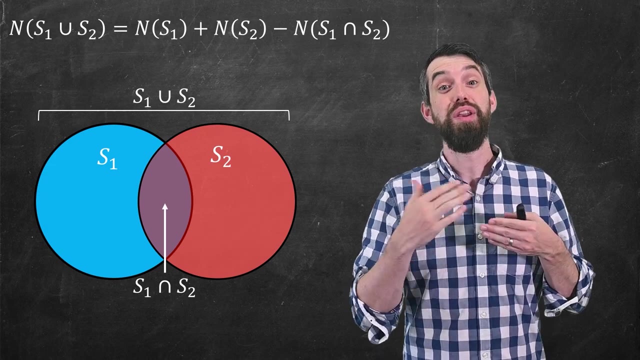 of elements in either S1 or S2.. And then what the formula says this is equal to is: well, it begins by taking the number in S1,, it adds to that the number in S2, and then it subtracts the ones that are in the intersection, the ones that are in both. It subtracts the number in S1,. 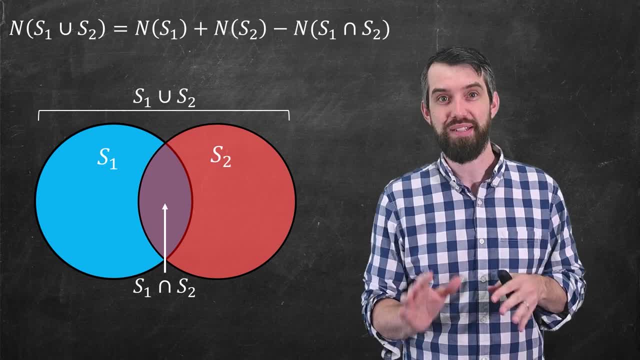 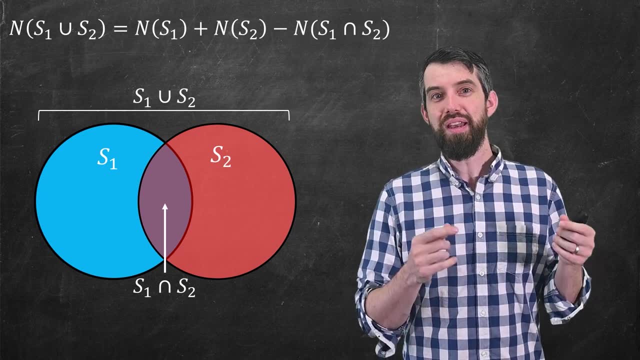 intersect S2.. Now I need to be careful about why this is the case. The idea is, if I just had the first two terms, the number in S1 and the number in S2, then elements in the middle would be double. 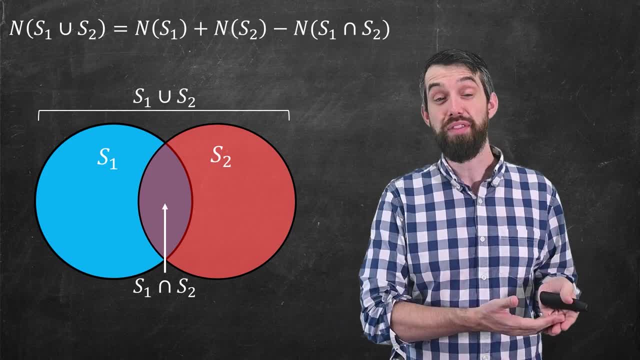 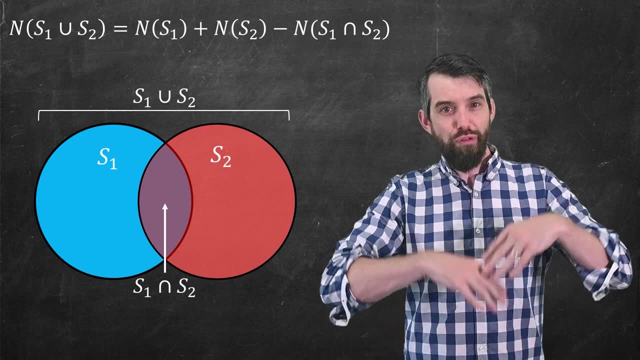 counted. They would have been counted when you added the S1.. They would have been counted when they added S2.. So you'd have too many in your count because of this double counting. So all of the ones that are in the intersection, all of the ones that are double counted, can be. 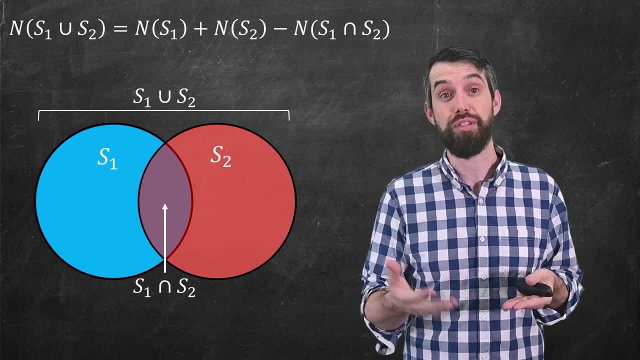 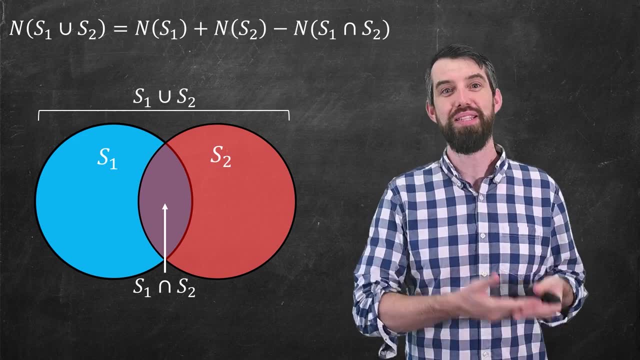 represented by the number in that intersection in S1.. S1 intersect S2. And as a result of that, if I subtract off this double counting, it now means that every element is counted exactly once. So you take the number in the S1,, you add it to the S2,. 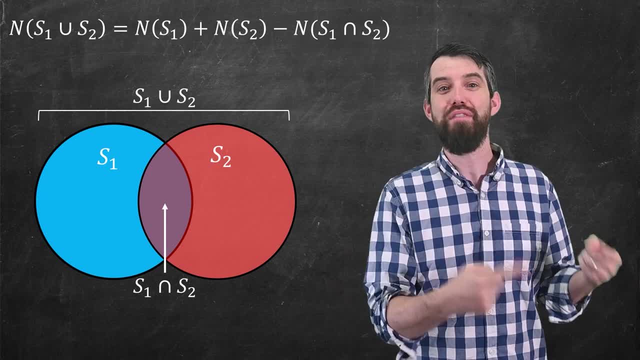 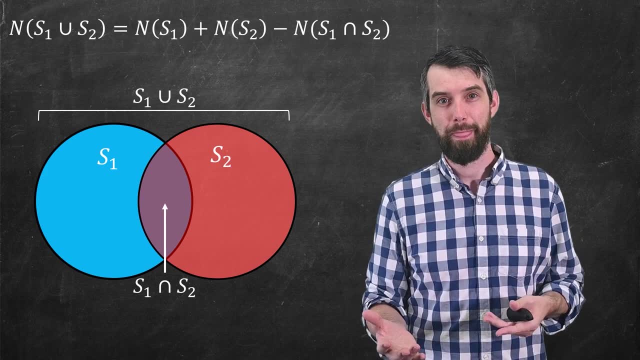 which means you have some double counting. but you subtract all of that double counting: the n of S1 intersect S2, and that just leaves every element being counted once. So this is my formula. Okay, so that was the double intersection problem. What about the triple intersection problem? So, 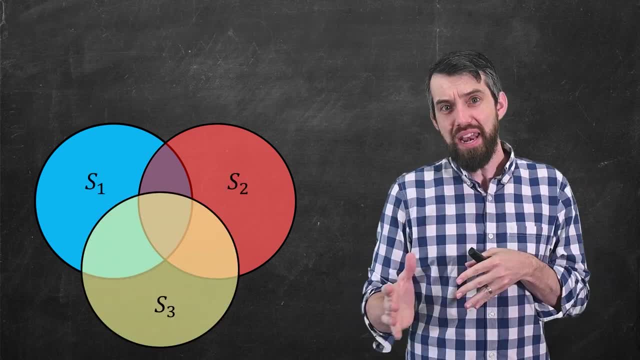 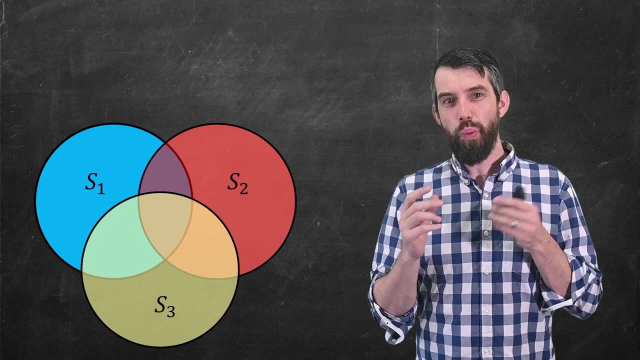 I've got an S1,, an S2, and an S3. And then I'm going to subtract the number in S1, and I'm going to be interested in how many are in all three of these, the union of the S1, S2, and S3. When 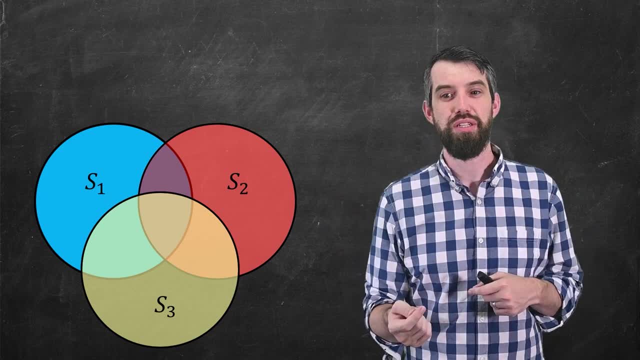 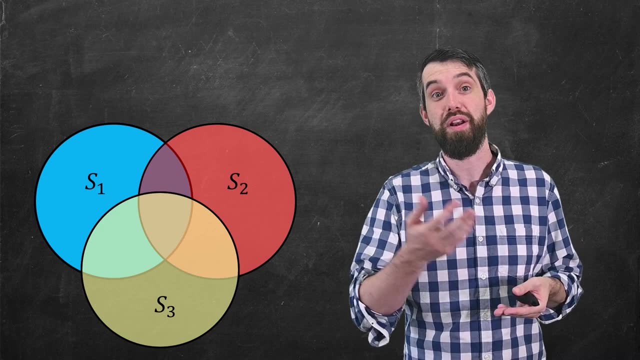 I look at this. there's some double intersections, For example the blue S1 and the red S2, they intersect and everything in the intersection can be written as the intersection of S1 and S2.. Likewise for S1 and S3, and for S2 and S3. There's a lot of different double intersections And then 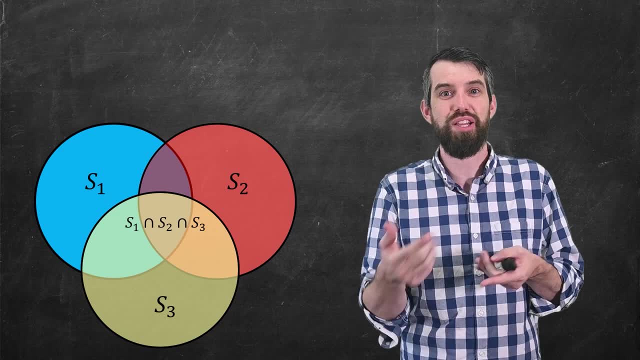 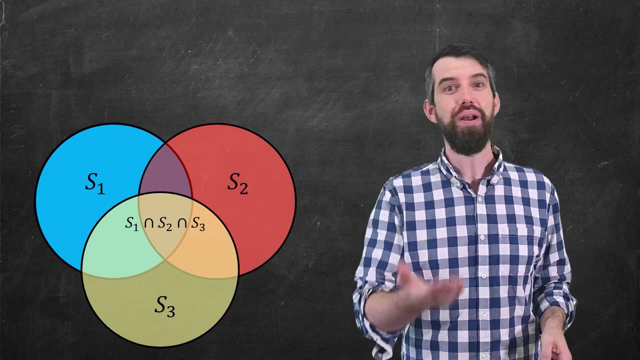 right in the middle is that triple intersection. These are things that are in all three of them: the S1 and the S3.. And then I'm going to be interested in how many are in all three of these: the S1 and the S2, and the S3.. Okay, so what should my formula be? I'm going to again begin. 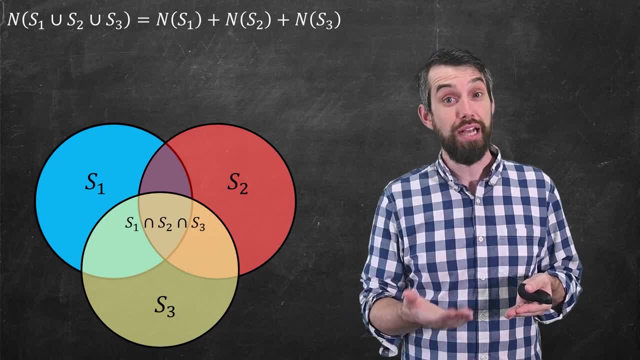 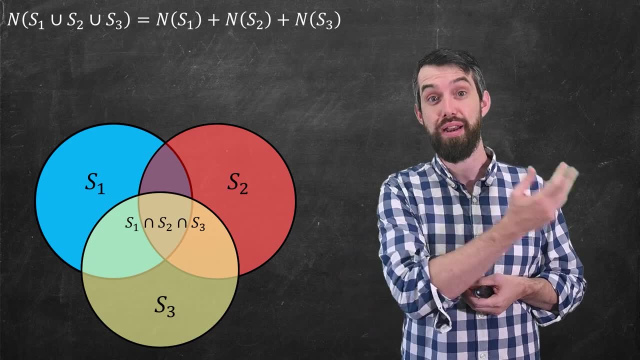 with the number in the union S1,, union S2,, union S3.. The first thing I'm going to do, I'm just going to add three different big steps: the number in S1, the number in S2, and the number in S3.. Yet we run into the same issue, which is that we haven't dealt with the 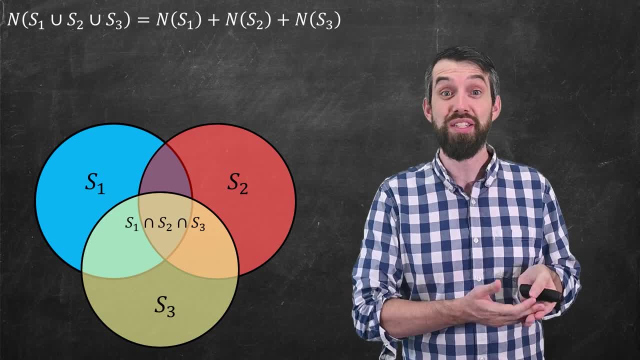 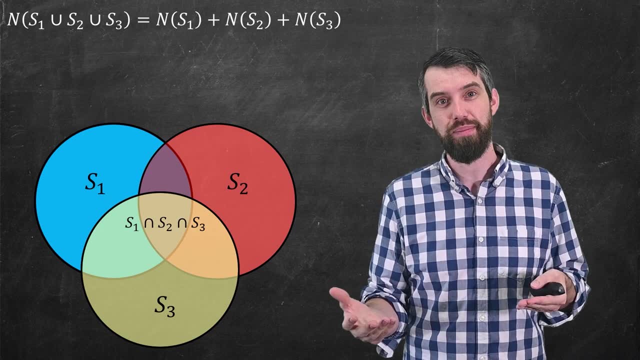 fact that some of these elements are double counted and in fact, ones in the triple intersection are being triple counted. They are part of the S1 and the S2 and the S3, so they get added up three times. So, following the previous formula, why don't I get rid of all of those? 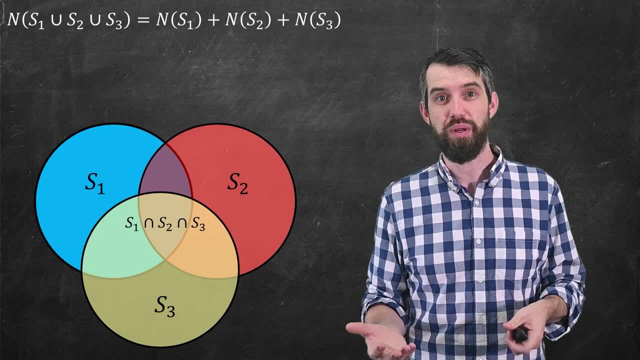 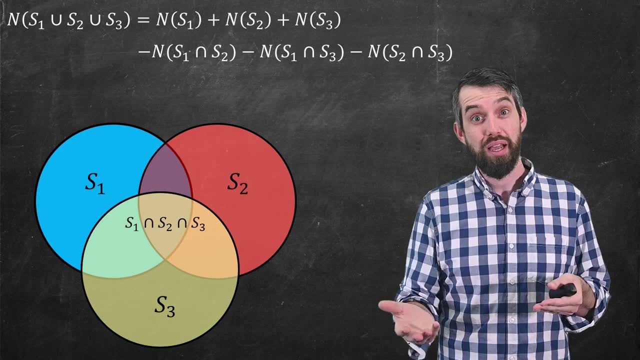 double counting all of those ways in which you could have an intersection between them. So I'm going to subtract three things. I'm going to subtract the intersection of S1 and S2.. I'm going to subtract the intersection of S1 and S3.. And I'm going to subtract the intersection. 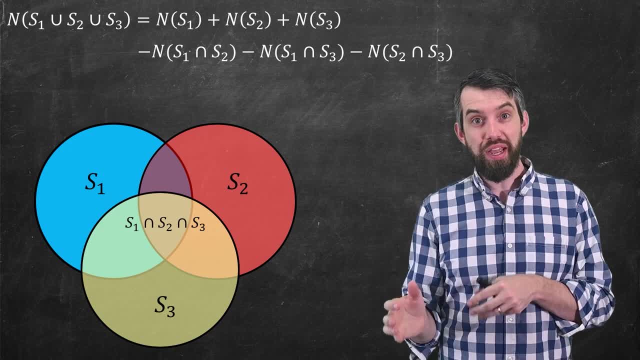 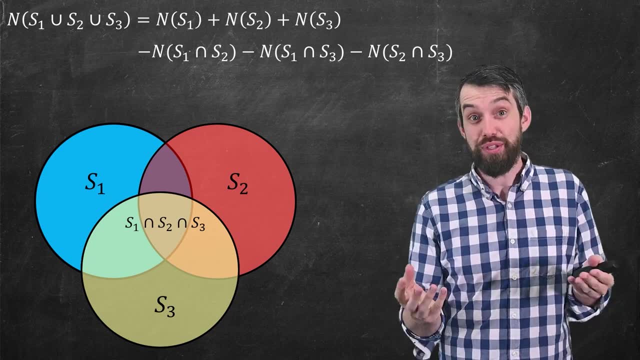 of S2 and S3. So this has gotten rid of any of the double counting where one element was in two different sets at once and so just adding up those sets would have double counted it. But now there's a problem. Imagine you're in the triple intersection. 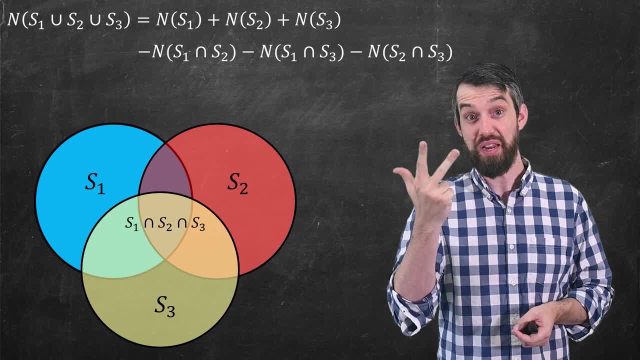 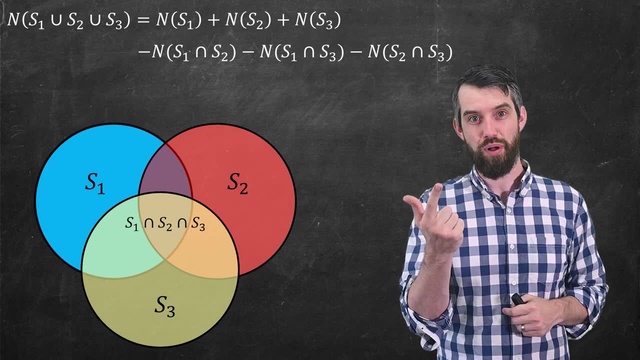 You get counted in the S1, counted in the S2, counted in S3. So you've been triple counted. But then for those elements in the triple intersection I then subtract off the one double where it's in it, I subtract off the other double where it's in it and I subtract off the. 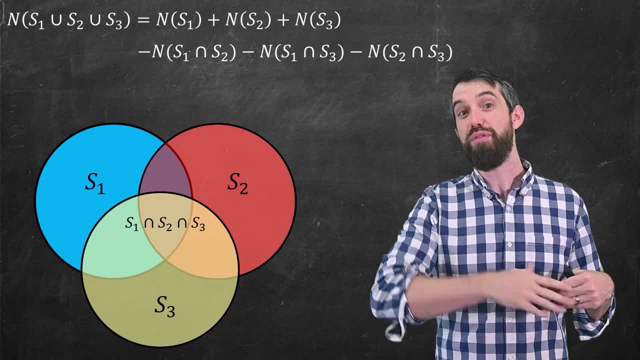 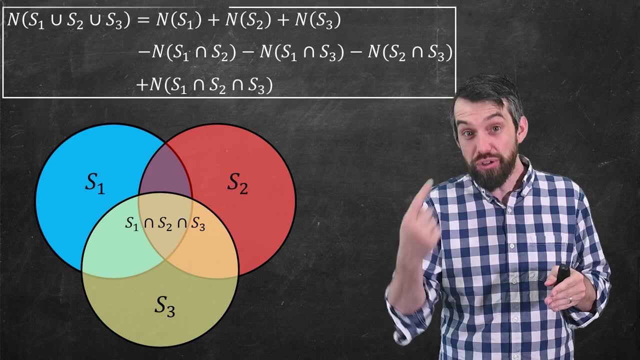 third double where it's in it. So things in the intersection got counted three times and then eliminated three times. Things in the intersection are not counted at all. I have to add back in n of the three sets to the S1,, S2, and S3. And so that is my formula. Now I don't encourage you to just